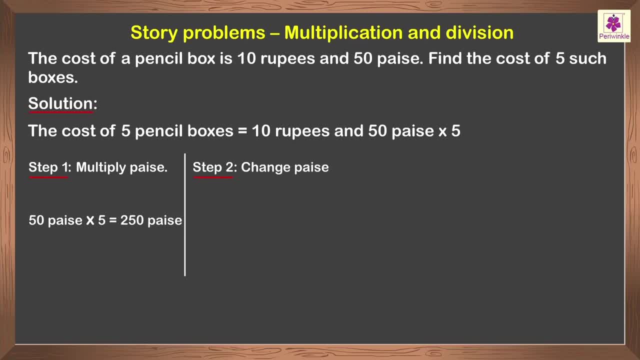 Step 2. Change paise to rupees and paise. Thus we get 250 paise is equal to 2 rupees and 50 paise. Step 3. Multiply rupees. 10 rupees multiplied by 5 is equal to 50 rupees. 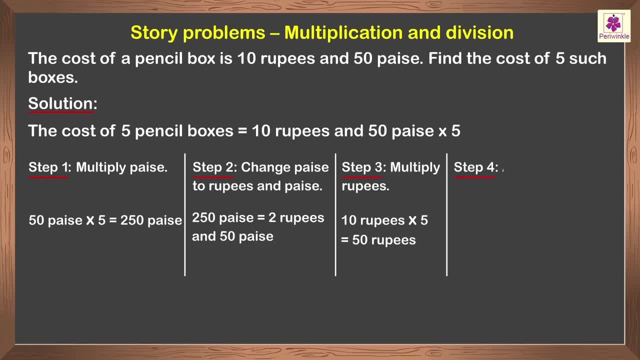 Lastly, step 4. Add rupees and paise from steps 2 and 3. So 50 rupees plus 2 rupees and 50 paise, That is, 50 paise multiplied by 5, is equal to 52 rupees and 50 paise. 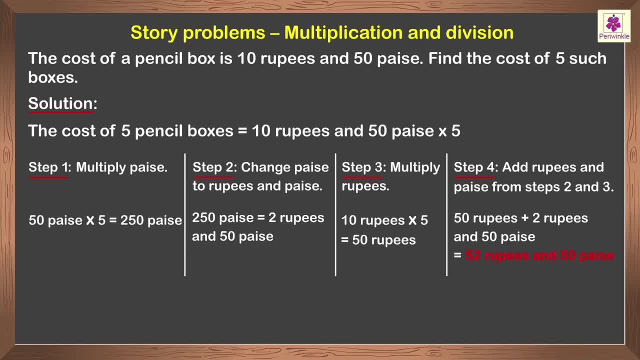 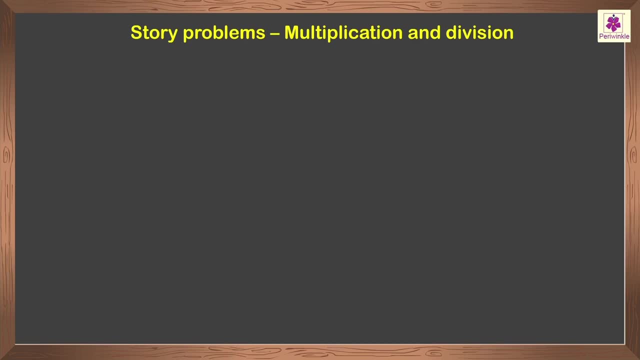 Look, we found the answer. Hence we say: the cost of five pencil boxes is 52 rupees and 50 paise. Now let us solve another story problem: 98 rupees and 50 paise is equal to 52 rupees and 50 paise. 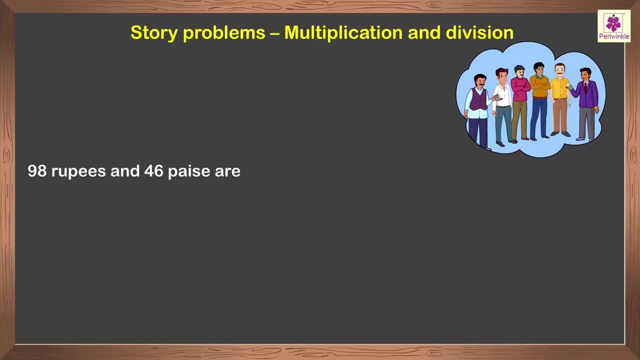 Voila, 98 rupees and 46 paise are equally distributed amongst 6 people. Now, in generally, the extreme increase in order of per capita is painters, and there is the such an issue in all martial art that the number ofもし this. 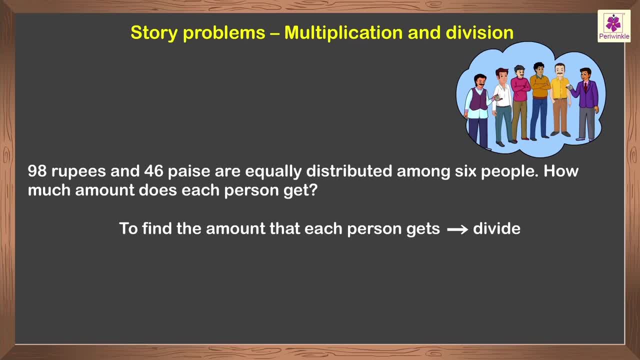 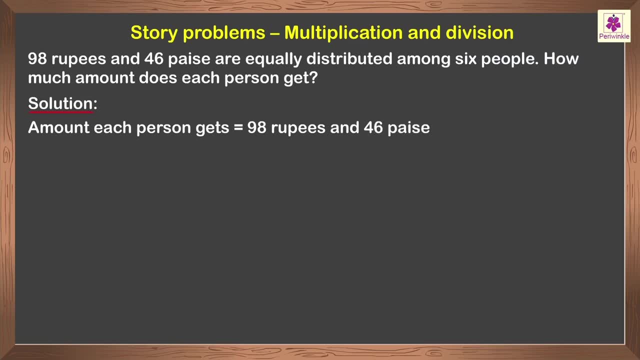 number x is equal to x fighting in the martial art and chess is equal to the number x fight in the Hong Kong Cessna. That is 98 rupees divided by 6. Any value of exactly☆? And anyways, the answer is-. 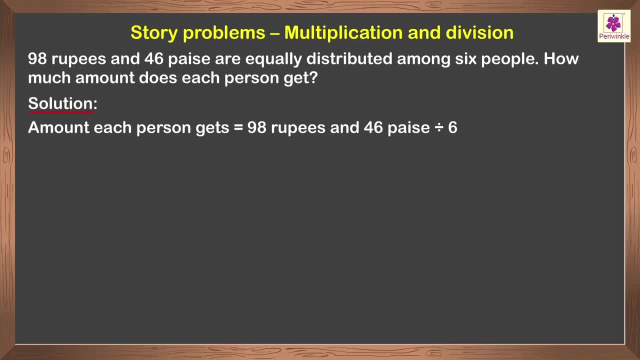 Commerce. Where is the change in order of feet? Now, to find the answer, let us follow a few steps. Step 1. Divide rupees. So, on dividing 98 by 6, we get 16 as quotient and 2 as remainder.